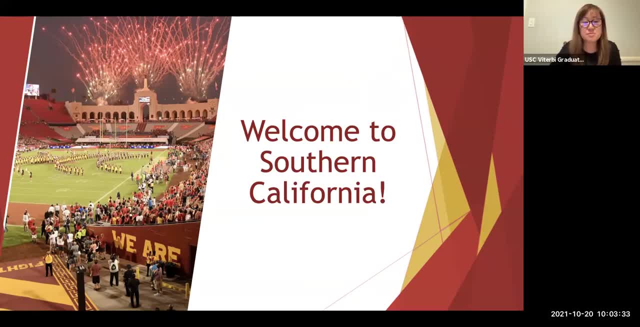 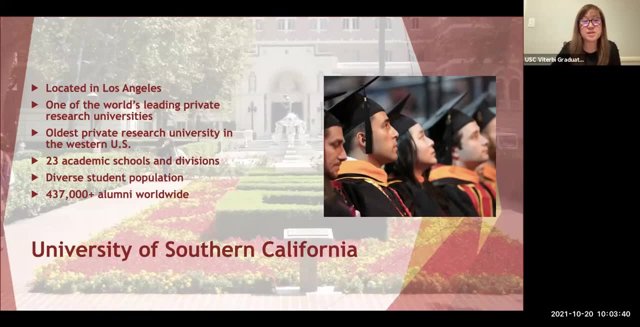 So they'll be speaking today about the new program and I'm going to talk a little bit about the university, The University of Southern California. most of you may know this. we're located in Los Angeles. The university, Oh sorry. 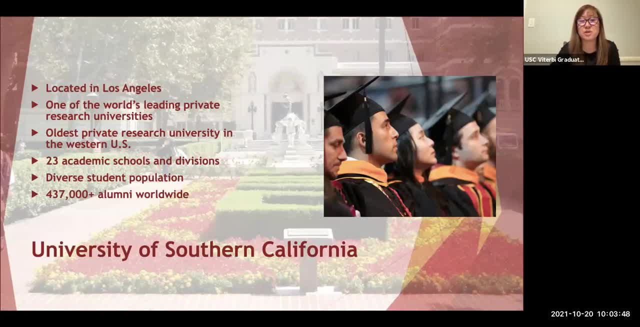 Is one of the world's leading private research universities and one of the oldest private research universities on the West Coast. There are 23 academic schools and divisions at the university, So, of course, in addition to engineering and computer science, there are also schools of business, communications, public policy, social work, school of medicine. 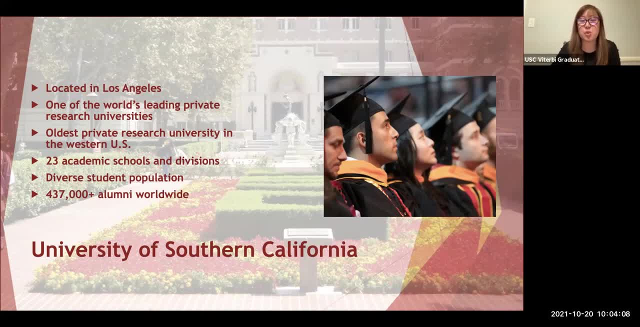 So you'll kind of see, as a student in the engineering school, we are very much advocates of interdisciplinary education and just kind of demonstrating how engineering really cuts across many of these disciplines. So you'll see a lot of collaboration between a lot of these other schools at USC. 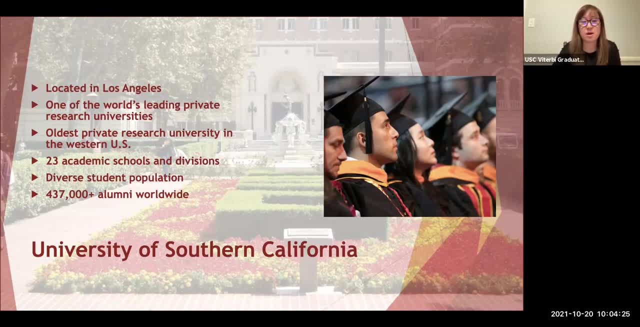 We have a very diverse student population, which I think is one of the best things about the university. There are students from over 110 countries that attend the university and it really kind of blends to the academic experience that you have while you're here. 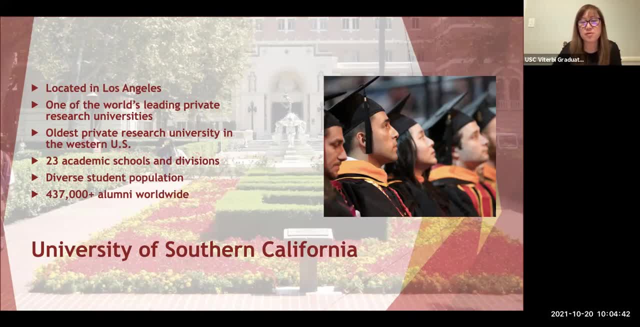 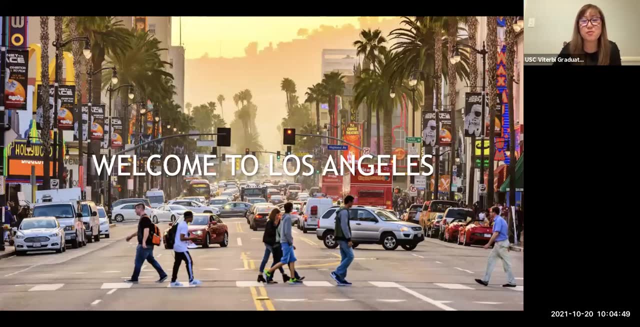 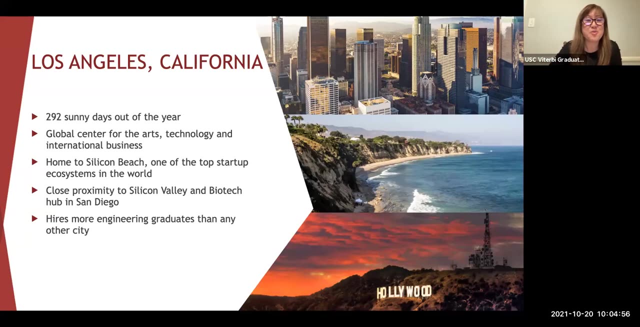 There's 437,000 alumni worldwide and about 90,000 of those are engineering alumni. Okay, So many of you may have been to Los Angeles before, maybe some of you haven't- but here's just kind of one quick snapshot of LA. In Los Angeles we kind of laugh- pardon my dog here. we kind of laugh because there are about 292 sunny days out of the year. 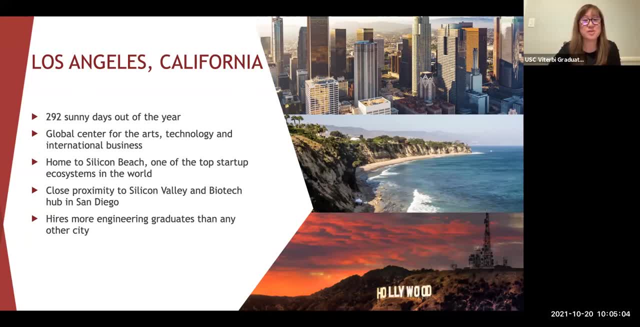 We are a global center for the arts, technology and international business. Sorry, give me a second. Okay, We are home to Silicon Beach, one of the top startup ecosystems in the world, and I'm close proximity to Silicon Valley and our biotech hub in San Diego, and many of you may not know, but we hire more engineering graduates than any other city in the United States. 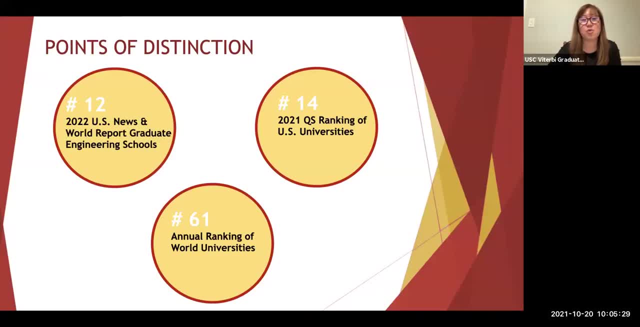 Okay, Okay. so a little bit about the School of Engineering. we're ranked number 12 by the US News and World Report, number 14 in the QS ranking of US universities And the number 61 in the annual ranking of world universities, which is the report put out by Shanghai Jiao Tong University. 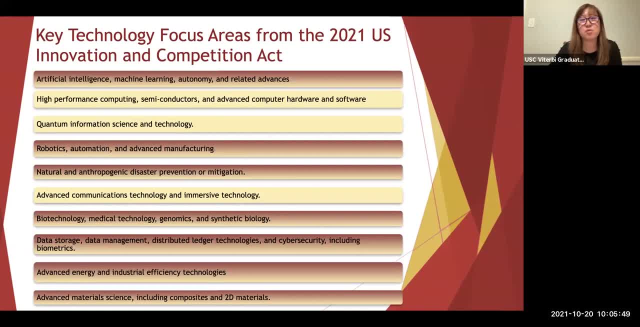 Okay, a couple of other items too. There was recently a US Innovation and Competition Act, and here are some of the key technology focus areas, And just one thing to highlight is that USC and the School of Engineering are doing a lot of research in many of these areas. 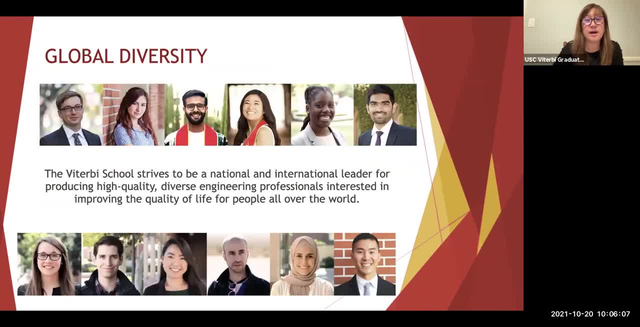 So I'll kind of have you take a look at that. And then I've kind of talked about the diversity of our school. We're really proud of the fact that in the School of Engineering we have over students from over 70 different countries that attend and enroll at USC. 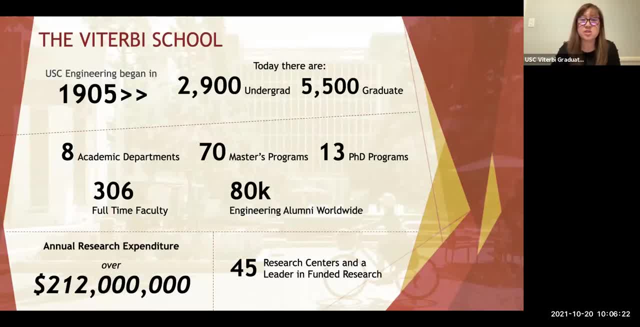 And then lastly, before I kind of turn it over to our professors, this is just a quick snapshot, by numbers, about the Viterbi School. USC's engineering program began in 1905 and we have a pretty sizable student population with 2,900 undergraduate students. 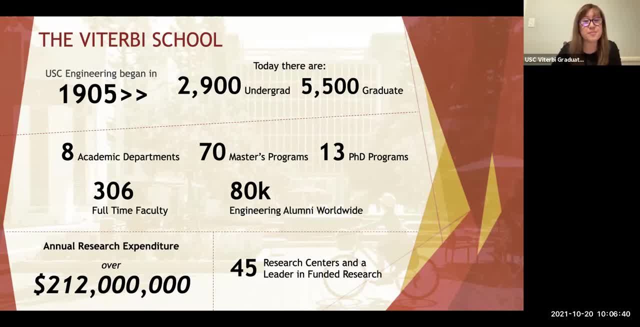 And that's master's and PhD. eight academic departments with 70 master's programs and 13 PhD programs. Okay, so that's just a little bit about the School of Engineering and the university And, if we don't mind, I'm just going to go ahead and turn it over to our professors, And please just let me know along the way if you need me to do anything during the course of your presentation. Okay, so I'll stop sharing now. 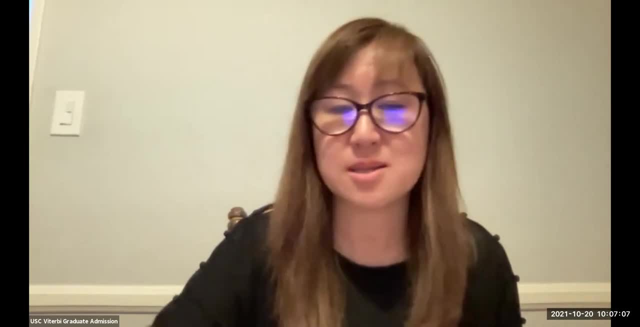 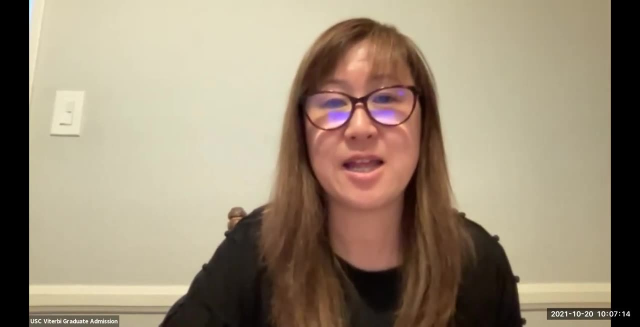 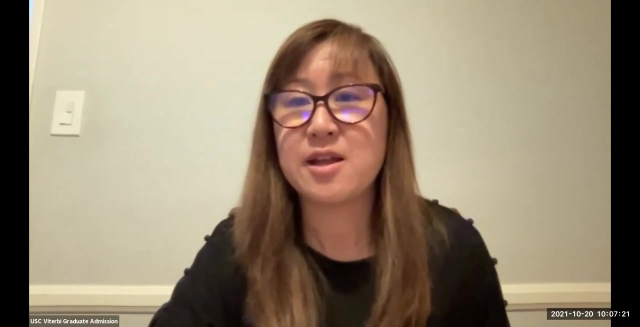 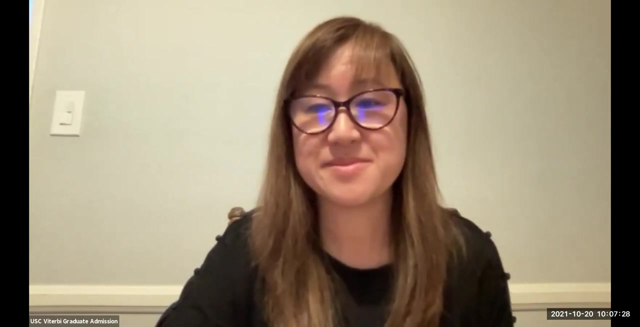 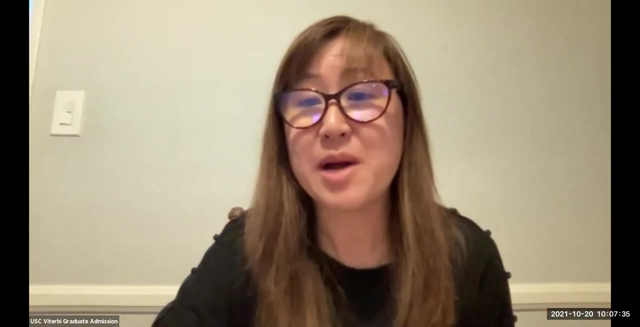 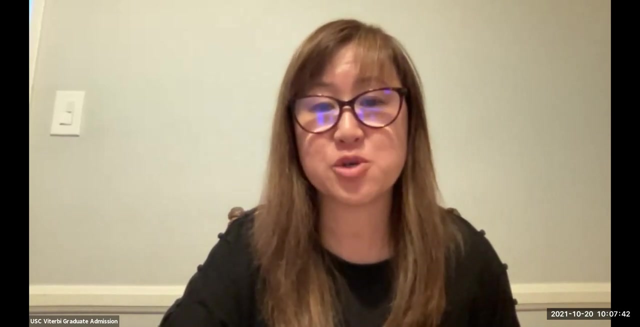 Pardon me, because I'm working remotely and I have a dog that's a little bit grumpy here. Okay, You're muted. I'm going to go ahead and turn it over to the three of you. I'm not sure if there's anything you need me to help you with to facilitate your presentation, but I can certainly do that. 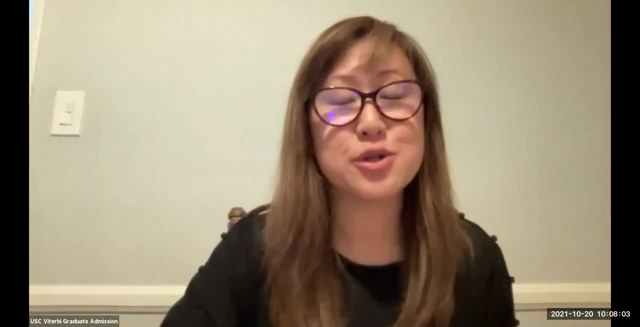 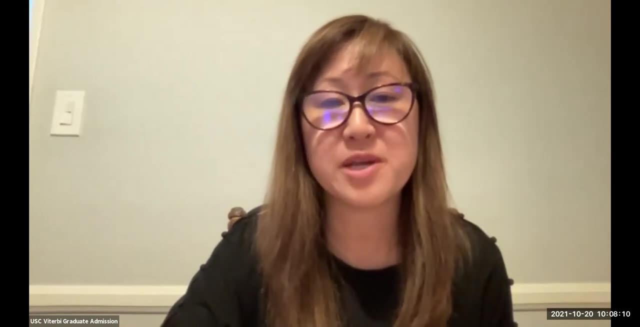 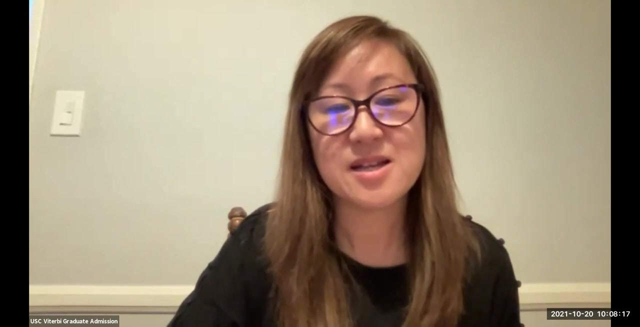 Okay, do you want us to start the presentation, or are you starting because we're not? Okay? Sure, I've actually ended the the introduction part. Did you need me to pull up the slides that we had prepared, or did you have? No, that will be fine. It just says we cannot share video, because he said he has been stopped by the host. 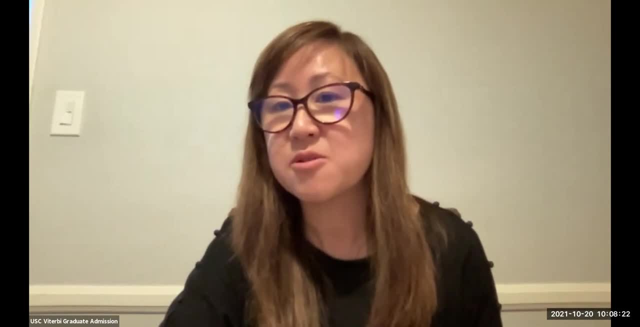 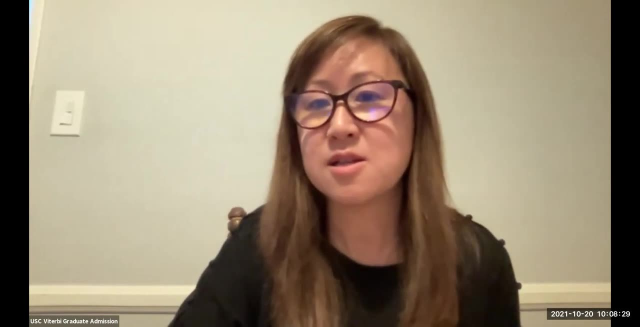 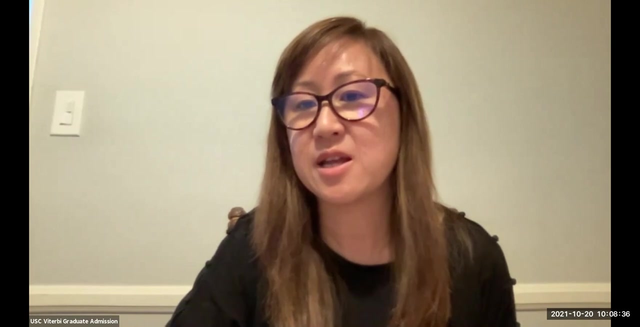 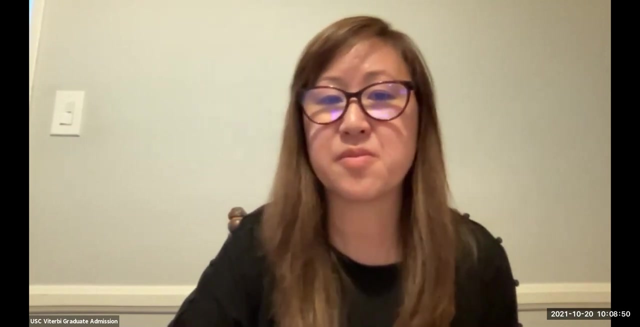 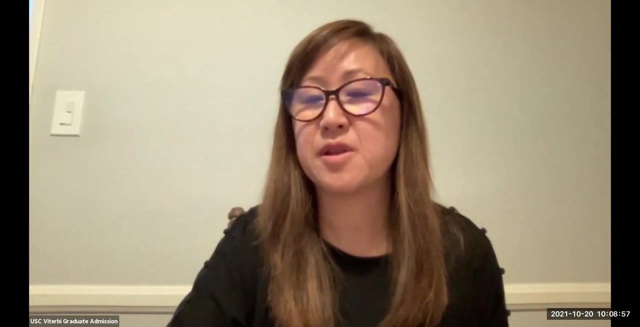 Oh, okay, Let me see. Did you need me to change your settings? It just says you can't start video because the host has stopped it. Okay, Sure, There's nothing I can see here, Just the fourth one. So why not? 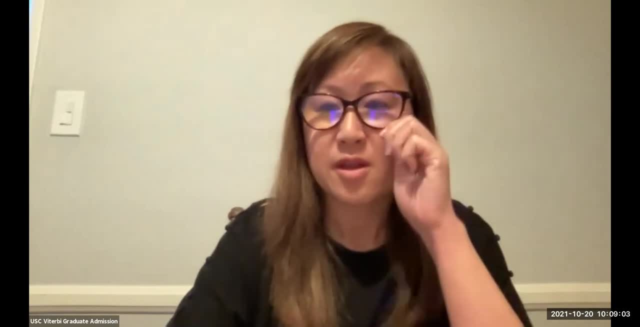 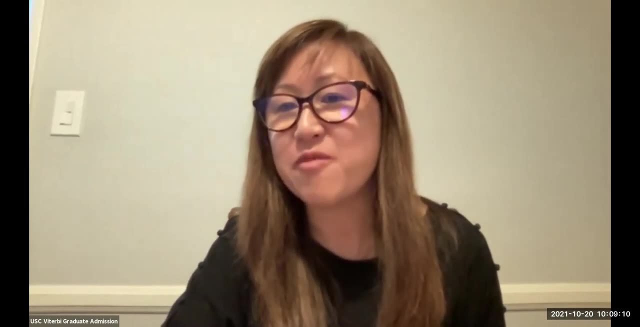 There's some holes down the top, That's right. there's no holes right there, That's right. Hey, hold on a second. Yeah, Yeah, Can you be there for the live? Yeah, I do not know how to turn your video on, but I've made you co-host to see if you can possibly turn your video on. 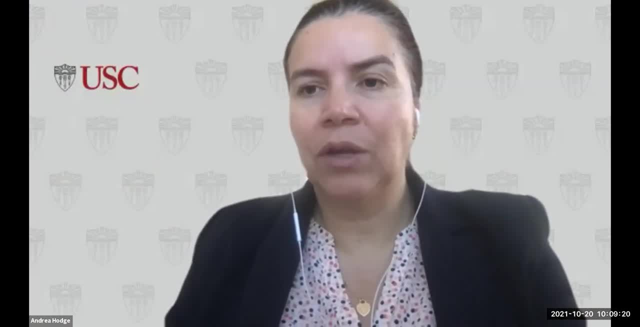 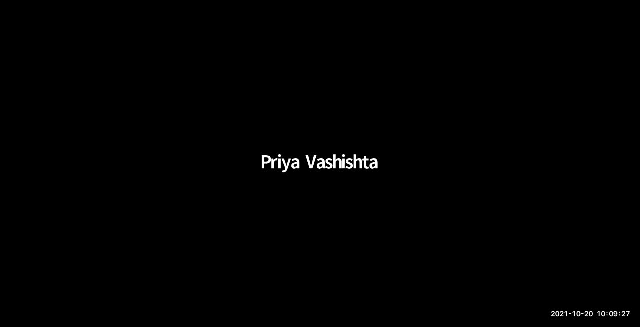 There you go. So that works. So that should work also for Kenichi and for Priya. Fantastic. So if we can have the presentation up, I think that we can, we can get started. OK, so shall we go through this PowerPoint slide. 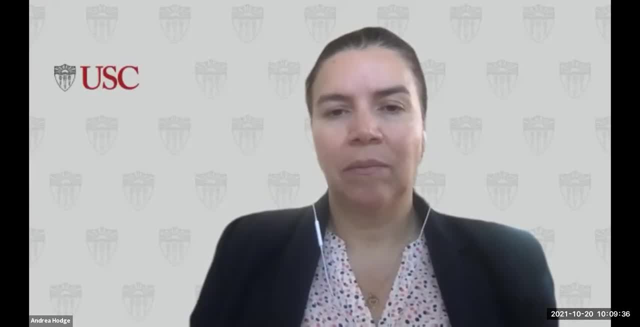 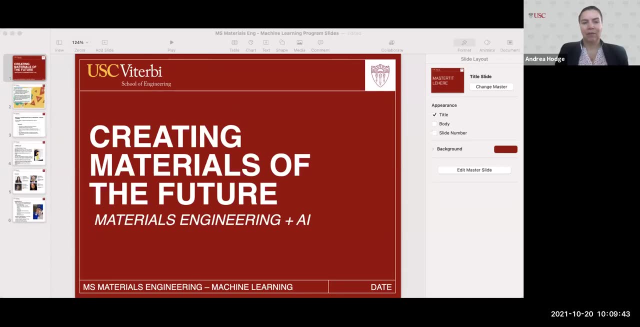 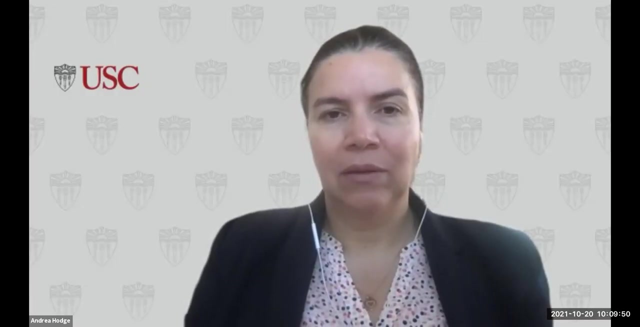 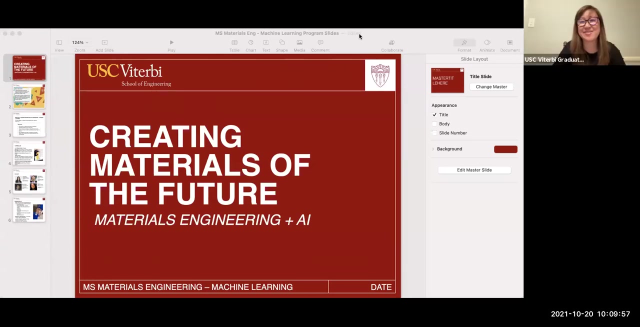 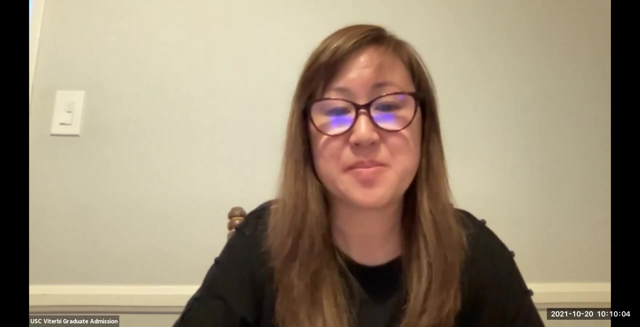 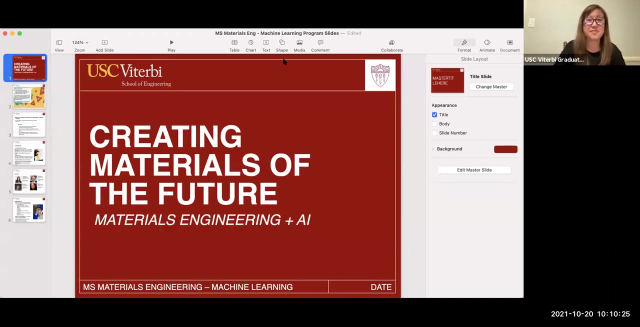 Yeah, she's going to put the presentation up. Yeah, you're muted. Give me a second. Sorry, I think it's not pulling it up. OK, let me see if I can do it now. Are you able to see it? 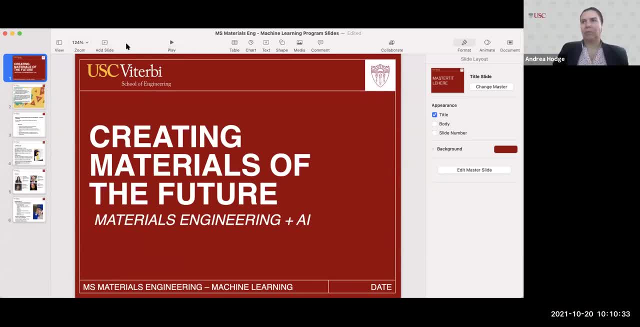 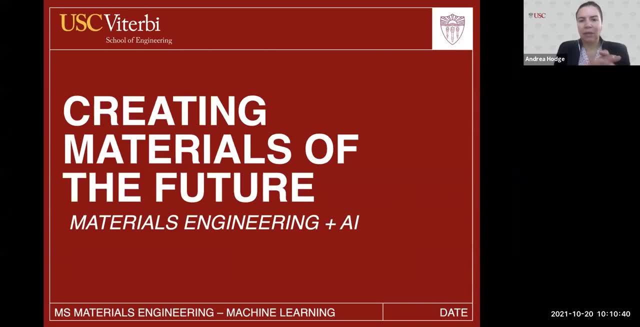 Yes, but it's not in presentation mode. There you go Now. it is So OK, cool, So let's get, let's get started. So again, thank you so much for coming for this info session. I am Professor Hodge. I am the chair of the Chemical Engineering and Materials Science Department. 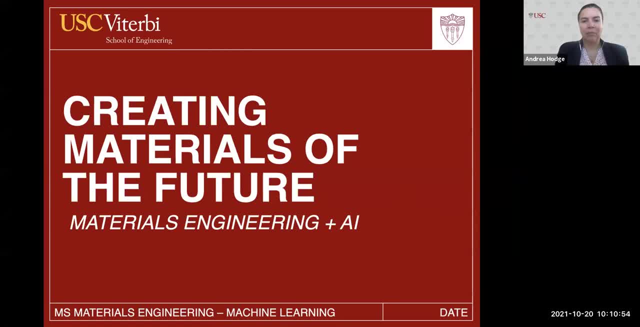 which is hosting this new and exciting master's program. So what we want to do today? really, we have two of them. One is a faculty who teaches the some of the classes in these new masters of materials engineering with machine learning, And so they will work. They will tell you a little bit more about the specifics. 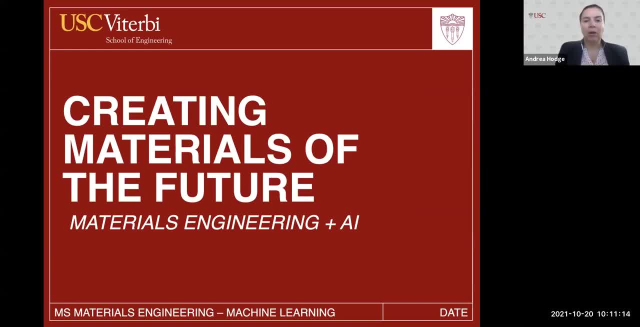 But we wanted to kind of give you an overview. The program has launched this fall And obviously for future applicants, you're able to join that program as well. So one of the main reasons this program was created is really to incorporate these new idea of 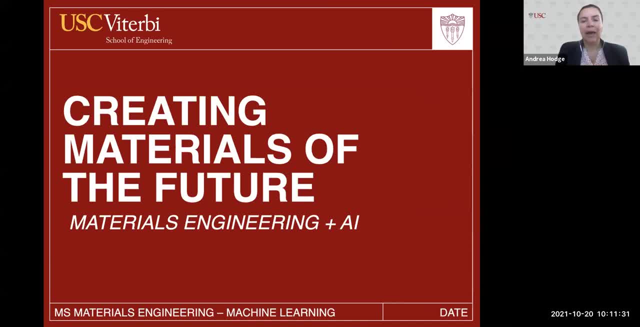 Emerging ideas of using AI and machine learning for faster materials discovery. So this is a specifically to materials discovery and material science. So, although there is a large component of computational component and machine learning component, it is with the focus of developing new materials, new structures. 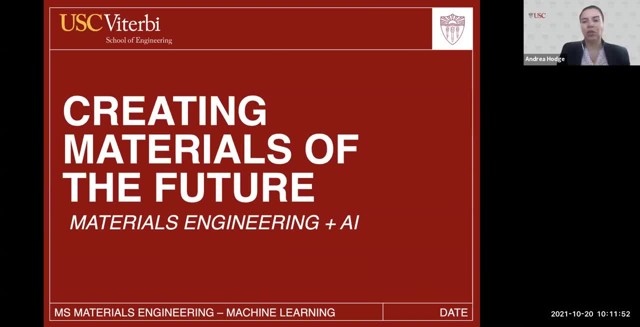 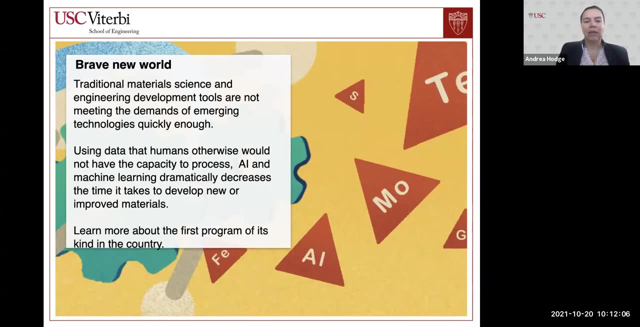 And that is why it's hosted under the materials engineering program here in the chemical and the chemical engineering material science department. So I think with that I'll go to the next slide. So again, as I was saying that the there is a need for faster materials discovery, 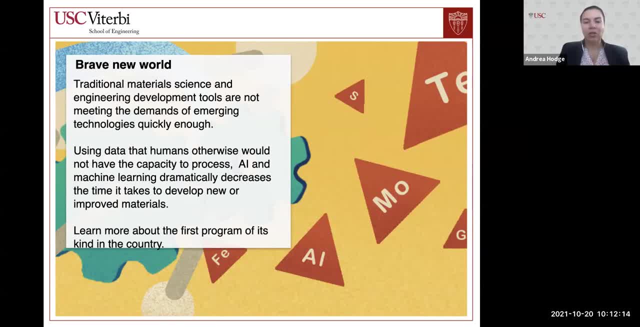 Nowadays, there's also techniques and machines available to do so, And so we are the first program in the country that is really starting to take tackling these challenges for materials discovery. As many of you know, many of the technological advances in any technology are directly linked to materials discovery. 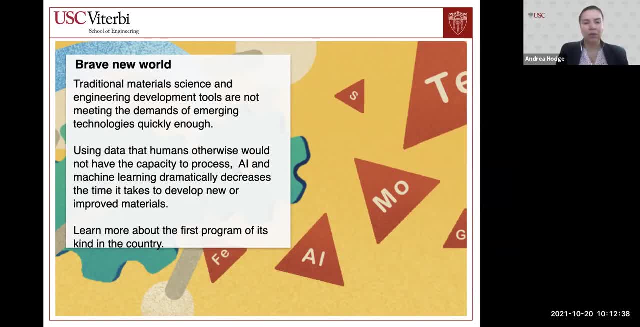 So if we're able to have materials discovery much faster and efficiently, then obviously these will improve all technologies overall, And this can range from, you know, polymers to ceramics, to metals and alloys, So this will encompass all different types of materials. 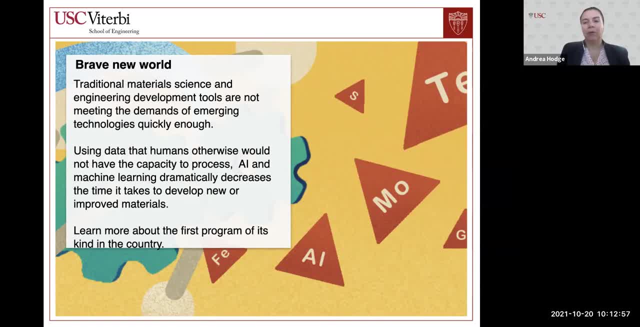 So what these machine learning program will allow us to do? you know, machine, a subset of AI, is basically using large numbers of data and data sets and data science in order to drastically decrease the time that it takes to develop new or improved materials. And so, again, this is the first program in the country. we super excited to launch this program this fall. 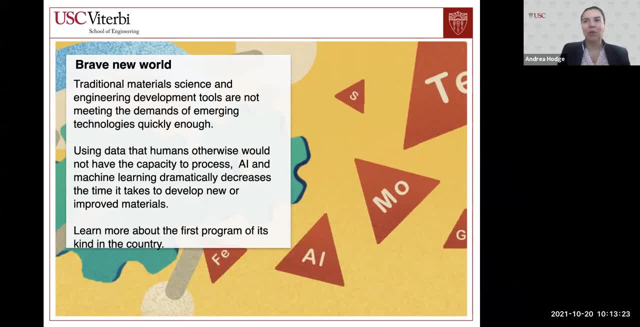 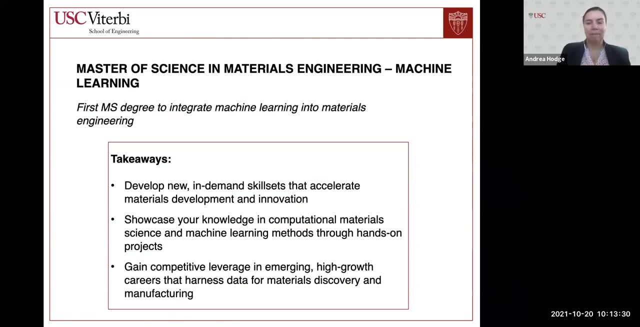 And so now I think I'll turn it over to Professor Priya Bashista and Professor Kenichi Nomura, that can tell you a little bit more about the specifics, Okay, so yeah, this is, like you know, really the first master degree integrating, like you know, machine learning, AI technology to, like you know, materials. 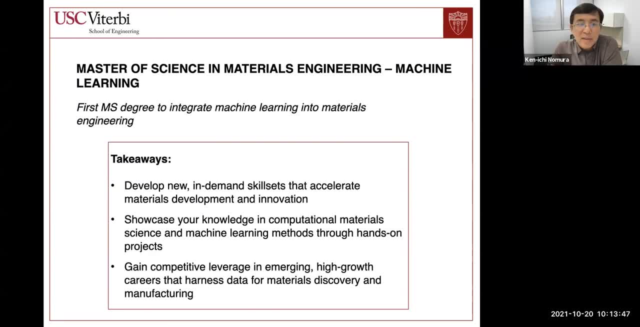 I think you know. so it's, it's very, like you know, new emerging field. Then the material development: historically, like you know, it's very long time, like you know, very expensive, right process But because of, like you know, this advancement, very, very rapid advancement in, like you know, AI, in the machine learning technology. 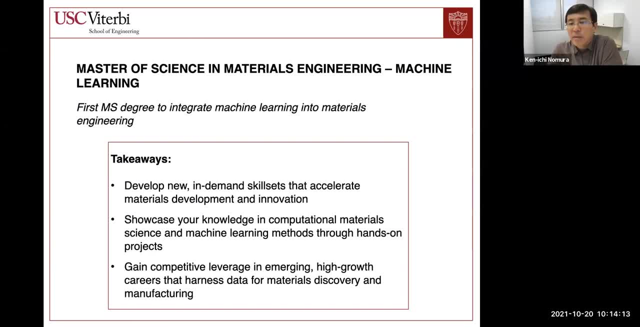 Now, like people are start kind of incorporating, like you know, this new technology to, like you know, material design discoveries For, like You know, many, many applications. It is sort of like you know, And then also like it's a new thing, so current, sort of like you know, that the curriculum doesn't cover this topic. 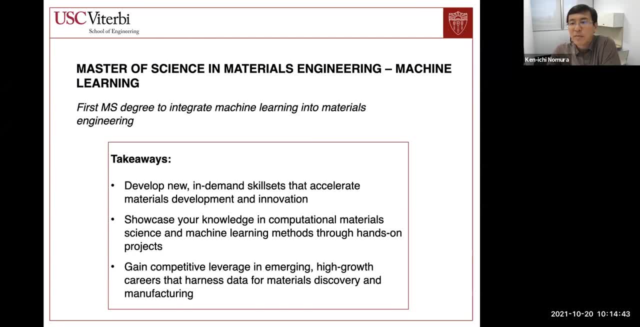 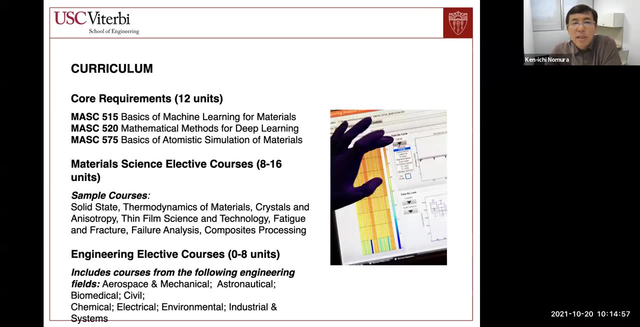 So that's why we thought like we really need to, you know, develop a new program weighing on this like a new field, emerging field. So can you go to the next slide, Kami? So here's a like kind of curriculum, a master program. 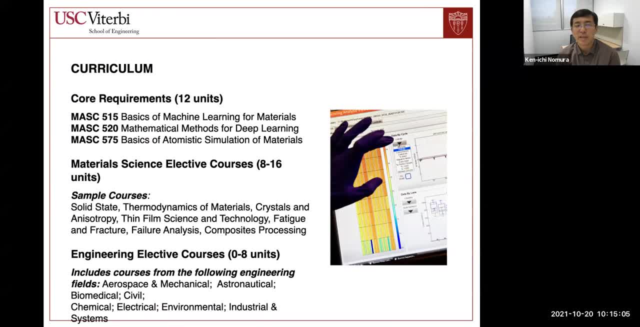 The name title is material engineering, with machine learning, which we have, like you know, three core courses. This, like you know, MSc 515, 520.. And this is, like you know, MSc 515, 520.. This is, like you know, MSc 515, 520. 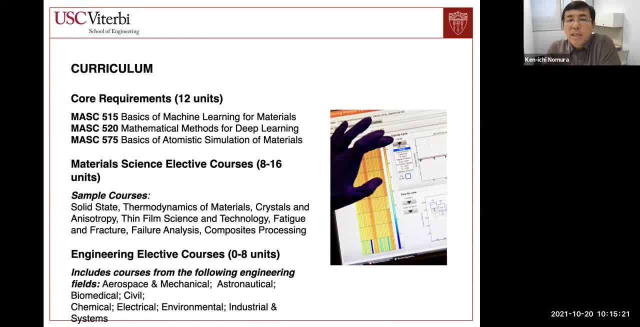 And this is, like you know, MSc 515, 520. And this is, like you know, MSc 535.. Which I can talk a little bit about. like you know, what you will learn from like each course is like, 515 is like a more sort of, like you know, focusing on like practical aspect of like this machine learning application for materials. 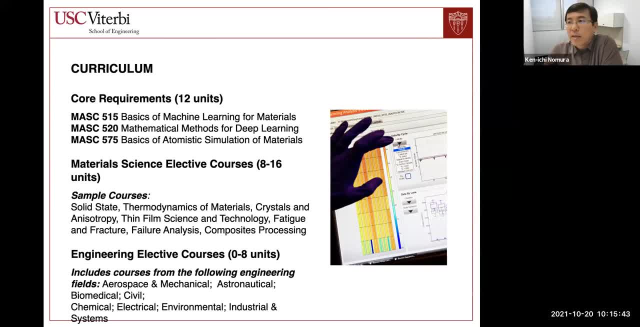 So we down like a basic concept, a little bit of, like you know, algorithm math, And then more on practical hands-on exercises using Python programming, Because that's also a very important skill set for nowadays. And then this 520 is more focusing. 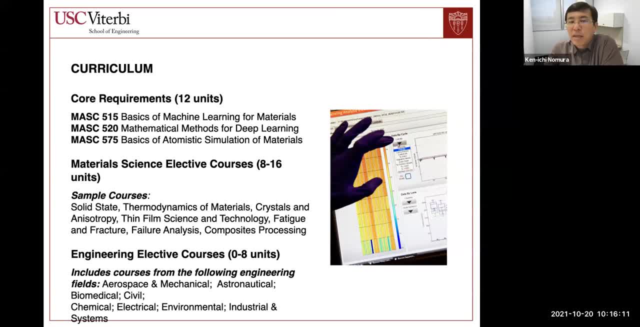 on mathematical method using deep learning technology. So we will discuss about what's the difference between deep learning, machine learning, AIs in each courses. That's something you will learn, But it's very, very important to have a solid understanding of math or theory. 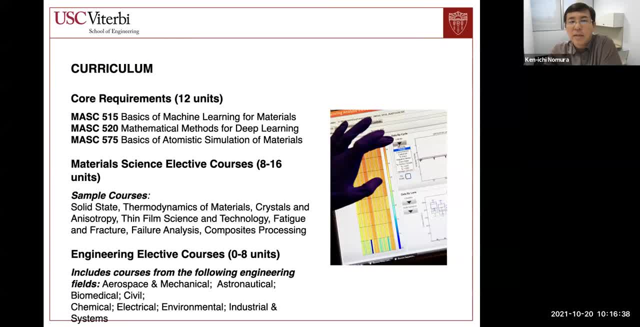 behind of this technology. So that's about 520.. And then 575 is again computational material, as modeling using atomistic simulations. So here you will learn how to use power of computers to model the materials. So USC has a supercomputer center. 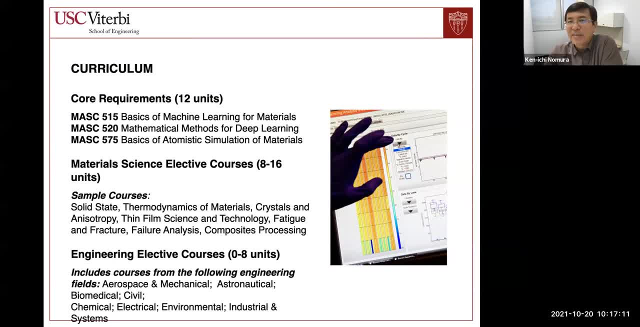 So each of you will have access to so many thousands of machines and then see how you can use them, And you can use this power to develop or design the new materials. So, Kenichi, can I step in to talk about this? So the core requirements, obviously. 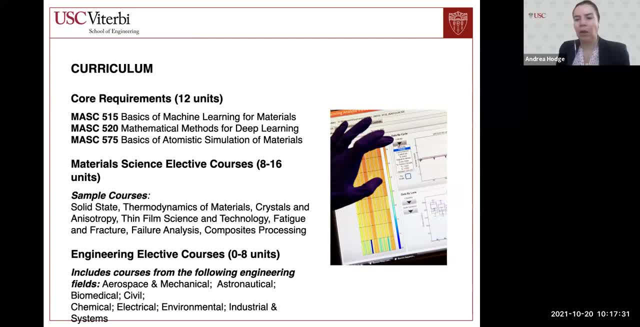 are heavily computational, which is part of what will allow you to develop these machine learning skills. And then, of course, because it is inside the materials program, the focus will also be to give you a fundamental understanding of materials issues. So there will be the classical thermodynamics of materials. 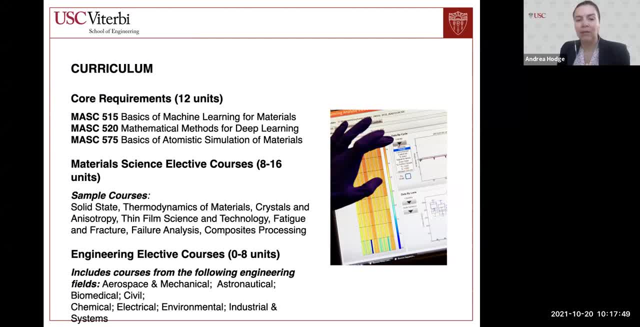 So you can take a lot of materials like materials, crystal, anisotropy, fatigue classes, fracture, composite processing, And so for those you can take eight to 16 elective units, So that means two to four classes, Or you can also tailor it to your specific needs. 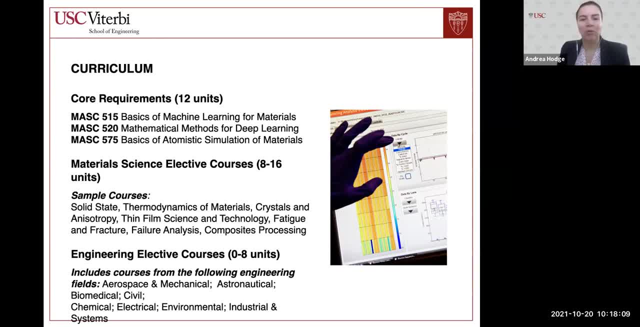 whether you're in a company or looking to start your own company or go back to academia. There's also engineering elective courses from various departments which have different aspects of the process. So there's a lot of different aspects of machine learning or synthesis or processing. 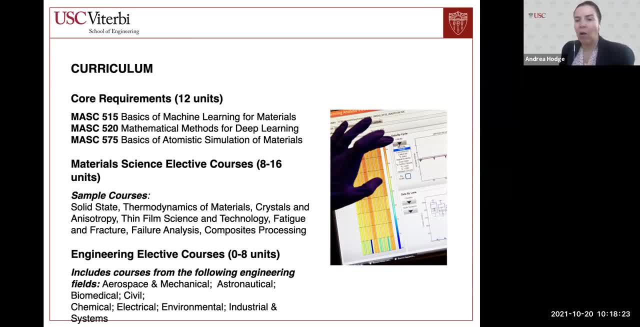 which can also be incorporated. So I think, overall, what Professor Nomura was also highlighting is that, in addition to having a strong computational background as well as the in-depth of machine learning, this will also allow to build a very strong material science core background which can be tailored. 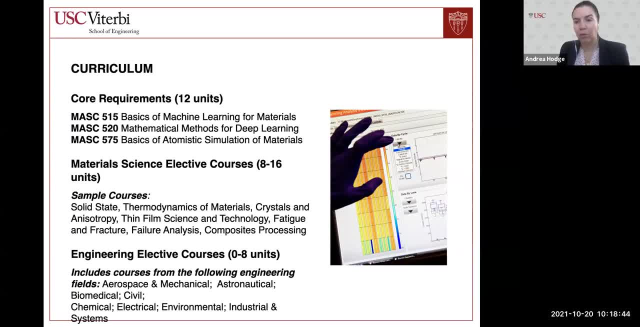 And I think this is key to having a successful master's program- is that you can tailor it depending on what you need. So if you're working on composites, you can take that as an elective. If you are working more in a mechanically focused field, 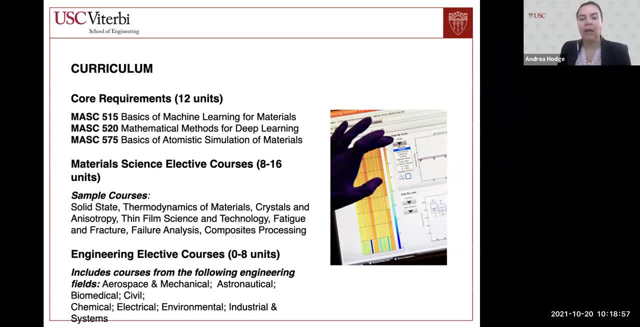 maybe you want to take something from the mechanical department Again, if you are more into large scale production, perhaps industrial and systems engineering will provide some classes. So the idea is that we provide the basics, We provide some requirements in order to also have basic, fundamental understanding. 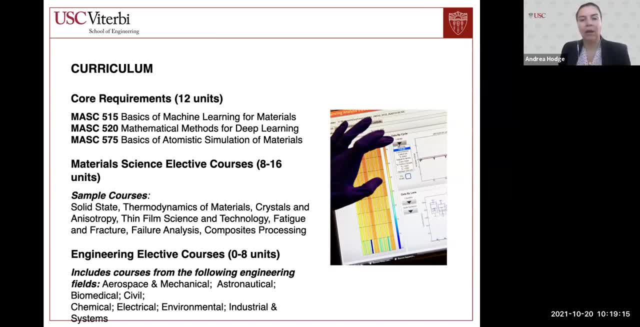 of materials but give you a lot of freedom to kind of tailor it to the specific needs that you have or your specific interests. So whether that be more apply and more general materials or more computationally driven, So you can kind of drive it and make the master's program directly tied. 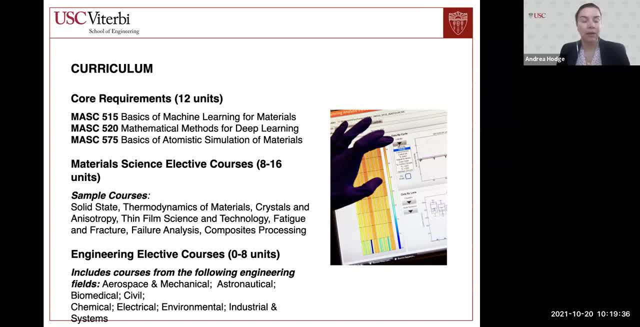 to your specific needs or learning desires. So again, the core is there and everybody will have to take that. The material, selective courses- you can take two to four, And engineering courses- you can take zero or two classes, And these would allow to really have a very tailored experience. 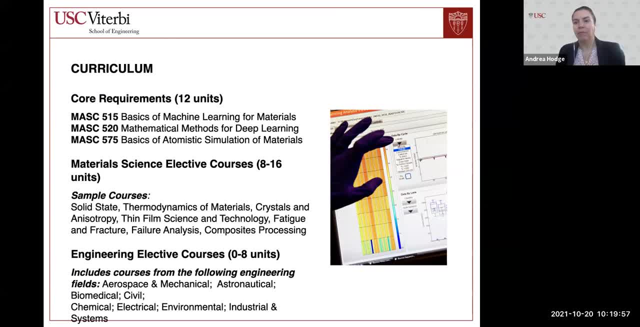 focusing on the things that you're really interested on. Yes, So this particular, this new program, yeah, as Dr Hoss said, it's very flexible. You have computational courses as a core But, as you can see, we have two kind of like. 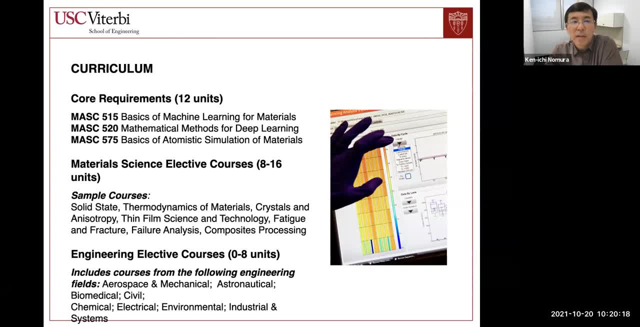 you know different elective courses, And then each one focusing on, like you know, more materials aspect or, like you know, more engineering aspect. So it depends on like you know what you like to you know which area you like to go after, like you know this master program. 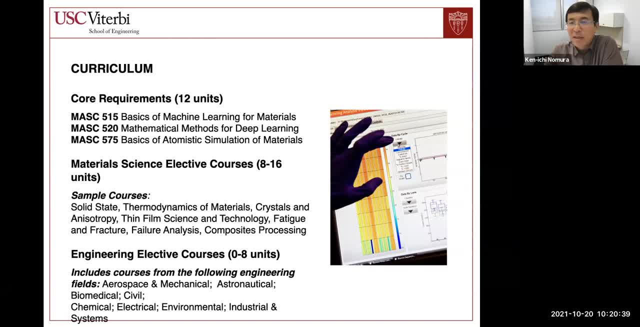 You can really tailor like you know, depending on, like you know, your needs. So Just to you know, as a logistic: So the total number of, like you know of unit requirement is 28,. right, 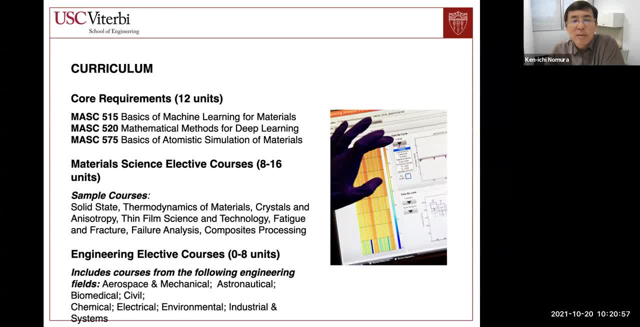 And so the core course covers like 12 of them. So you need to have, like you know, 16 more, And then you need to take like 8 to 16 from this material science electives, And then the engineering elective you can take, like you know, up to 18.. 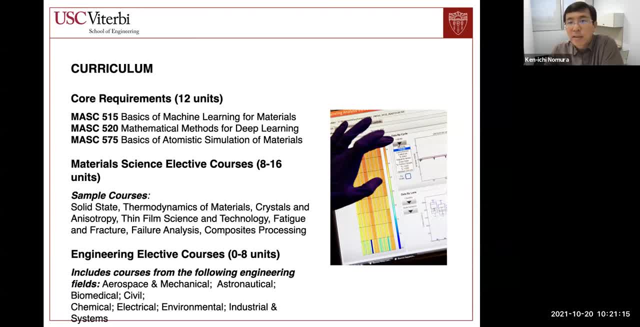 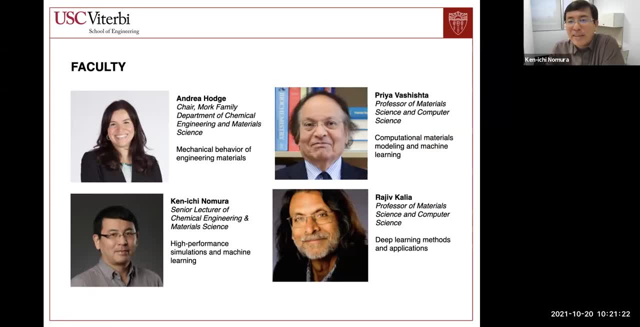 So Maybe next slide. So these are our faces, I think we introduced, like you know, Dr Andrea Hotch is the chair of, like you know, our department And Dr Priya Basishta, who is in this session as well. 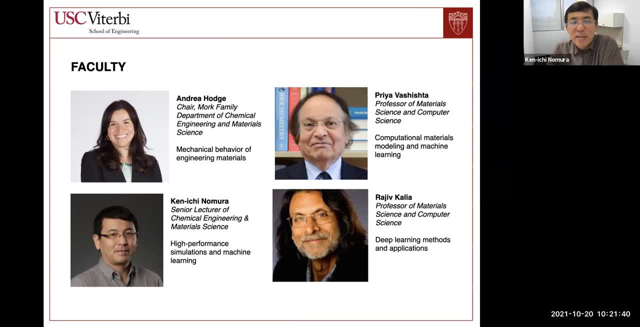 And me, Kenichi Nomura. I'm a senior lecturer of, like you know, our chemical engineering, material science department, And also Professor Rajeev Kariya, who teaches, like you know, 520, the mathematical method. 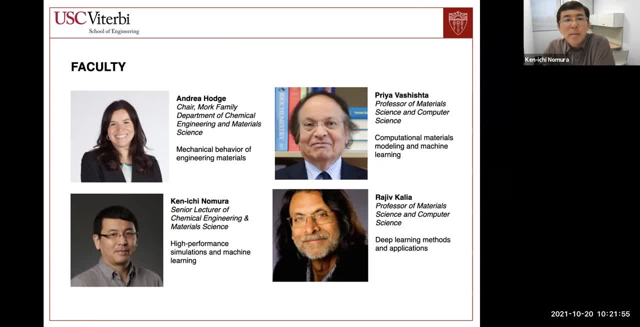 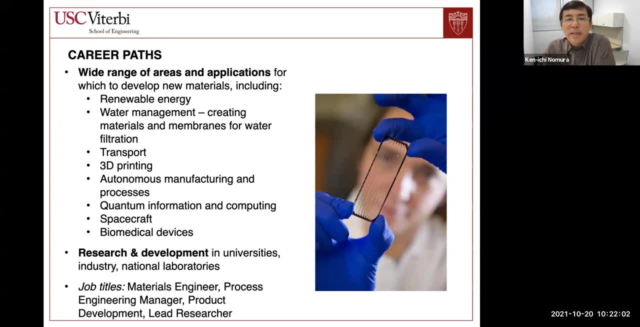 for equity planning. So this last slide is probably the most kind of- like you know, interesting for you guys. like you know, after you get this like degree and what you can do right, what kind of job, like you know, you might be able to get, 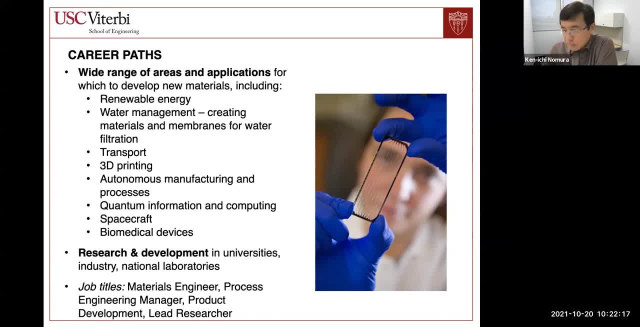 So, since, like you know, this machine learning, assisted material design discovery is, like you know, used, can be applied to any field, material field. So you could, like you know, do like, let's say, renewable energy, or, like you know, 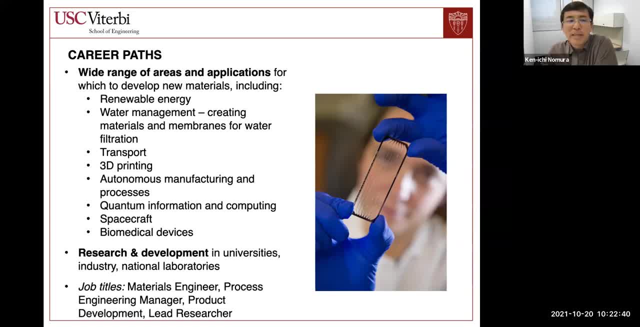 water management. And there is 3D printing, like you know, additive manufacturing. These things Also, you know, Yeah. And also, like you know, bio and the, you know, medical devices. Any field, this technology is in the high demand. 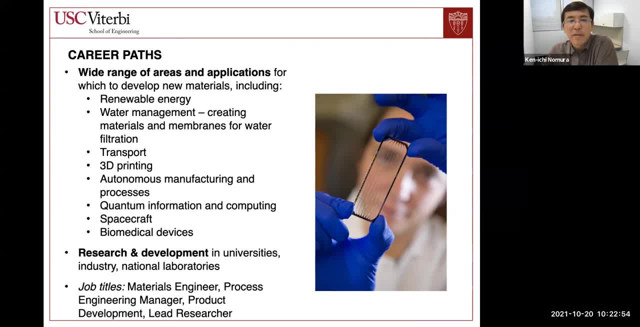 So I think these are, like you know, a field you can find the jobs after, like you know, master program. Also, like you know, it's really really hot research topic in academia, university, national lab, even, like you know, research department in the industry. 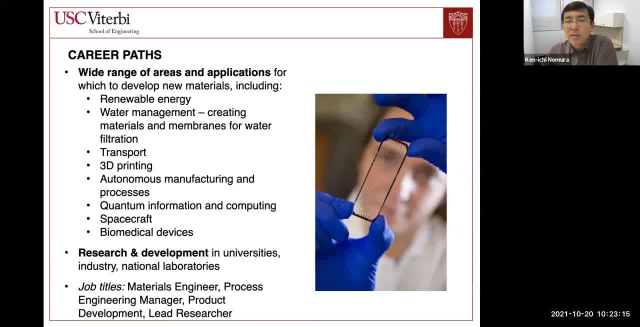 So that's also like you know, Yeah, And also you know the job opportunities in this kind of like you know type of jobs: Job title design- Yeah, I'm not sure These are like you know. I think we can find from like a, like former student or 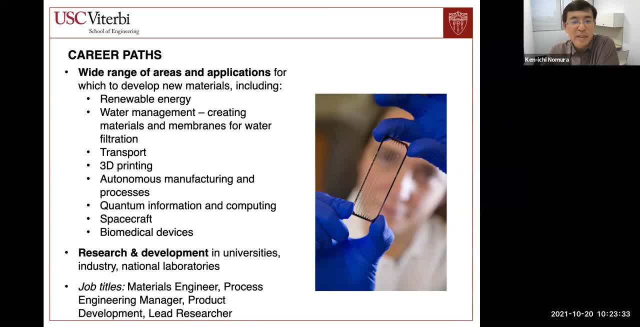 like you know, the online, like job opening related to, like you know, this field. So, Priya, would you like to step in and say, uh, no, i, i for a perspective, i. i think i think what all need to be said has been said between. 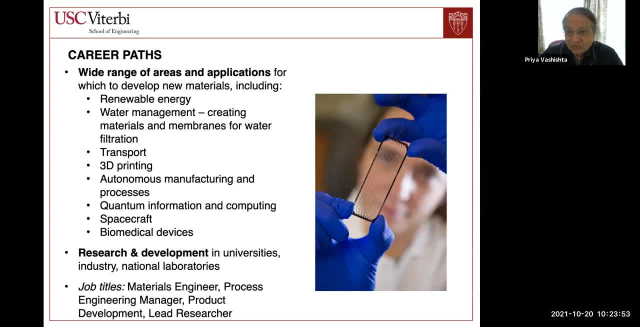 you and kenichi, so this is all good. so i i think this was, you know, a short presentation, kind of just to give you an overview of what's cover and what will be, uh, the required courses, as well as the flexibility of the program and some of the goals and objectives, which is really to give you. 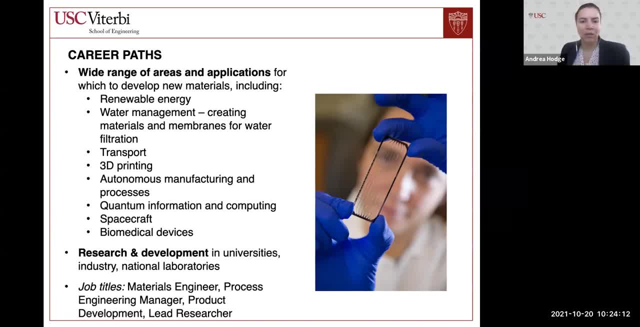 the tools to be at the cutting edge technology, while still while um for faster materials discovery and so and providing you all the tools that you need to be highly sought after for companies or graduate school, because this is the way that materials discovery is going to happen for a broad range of industries and research fields. so i think, with that um, that's. 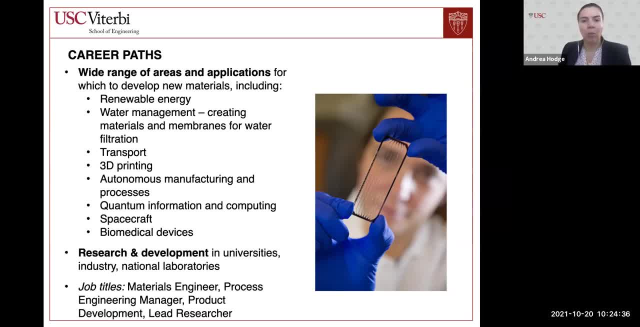 basically the end of the presentation and we are open for questions, more specific questions, now that we provided you an overview. thank you so much. professors. um, well, everyone um is welcome now to kind of put their questions into the q a window. um one question that um, maybe i can start. 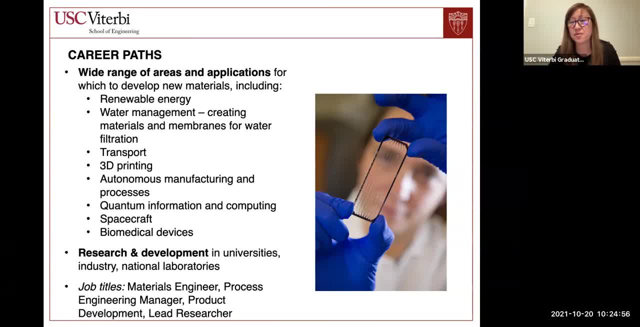 with, if you can um touch on that. i'm sure many um of the applicants are wondering that kind of: what are we looking for in a successful applicant and a candidate? what background should they have? just in, in general terms? um, could we kind of just touch on that just a little? um, i think, um in the general sense. so, materials, science, materials. 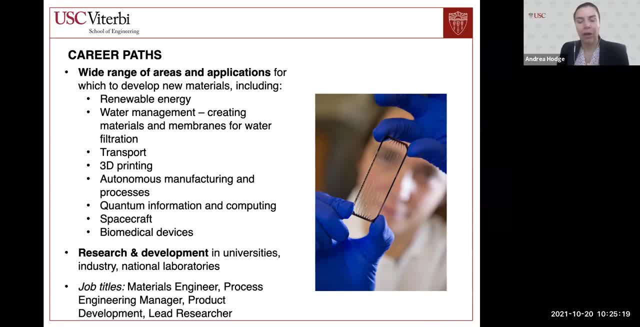 engineering is a very broad field regardless, so we always have students coming from physics, chemistry, other engineering fields, from material science fields, mechanical engineering fields. so you're looking for a strong scientific background in physics, chemistry, um mathematics, of course, but what we're able to provide by providing these core courses is that students will be able to learn. 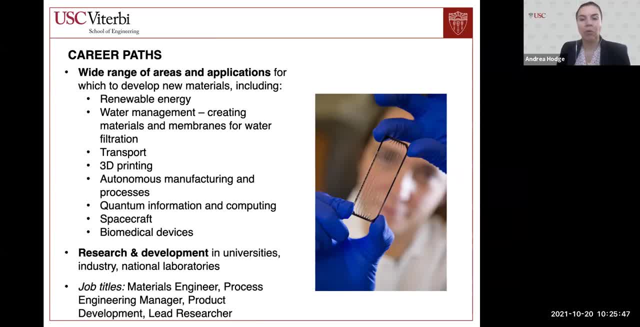 the basics of machine learning, as well as go several levels deeper and even farther if they want to take more computer cloud computational classes as the electives, i think. in regards to the computational classes, uh, perhaps priya or or kenichi can speak more about some additional. 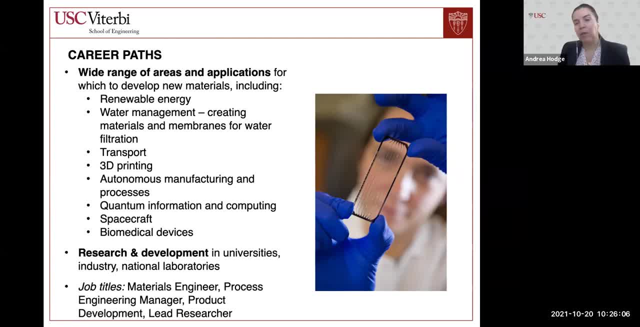 background for the, but for the materials part, it really can be from any field, either sciences or engineering. yeah, so i i always kind of, like you know, emphasize in my class that this is, like you know, a machine learning ai course. right, but you, you need to have a very 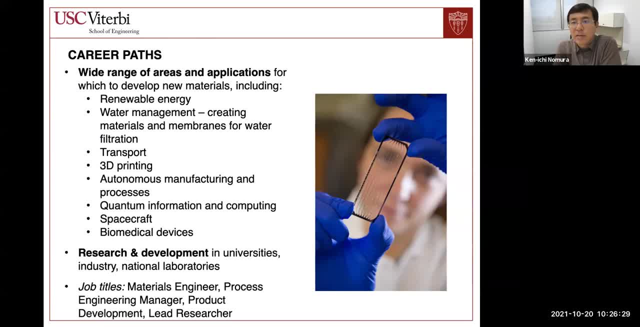 like you know, solid uh materials background, uh, material engine i mean. so it doesn't have to be like a material itself, but uh, you, you should have a very, very solid kind of like understanding and skill set of your own background. not like you know you, you are good at, like you know, writing a. 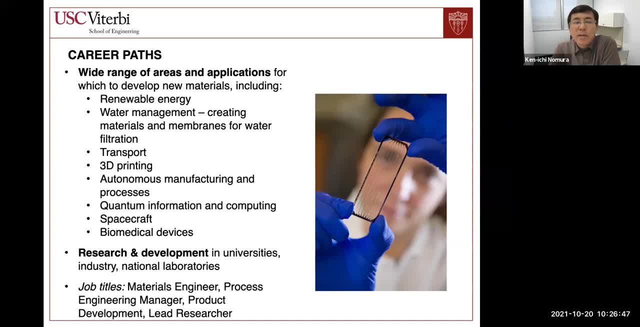 python code or something like that, because you see, like uh, um, a lot of, like you know computer science, uh, student, uh, you know uh, learning, like machine learning ais, but uh, would they be, you know, successful in this like you know our field? absolutely not, because they, they don't understand. 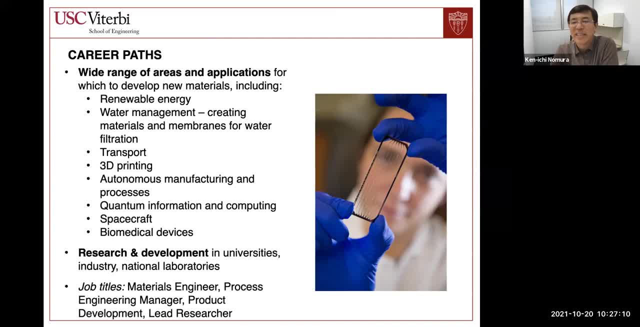 like they, they have no background of, like you know, materials, engineering, they they know, like you know, some programs there but they have no idea like how to you know apply to our field. so each of you, uh, you should, you know, uh, spend enough time sort of like you know, or deepen your like you know, knowledge and you know skill. 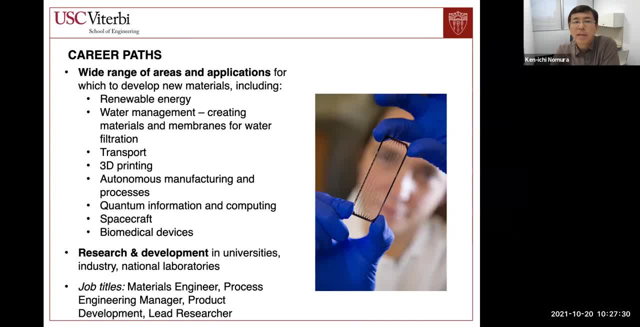 set uh for your background, then on top you can add, like you know, all this machine learning, like you know, technologies, that. so this combination like you know, of, like you know, your background, solid background with, like you know, machine learning, ai technology, makes really that difference, like you know, makes me really really strong, like you know. 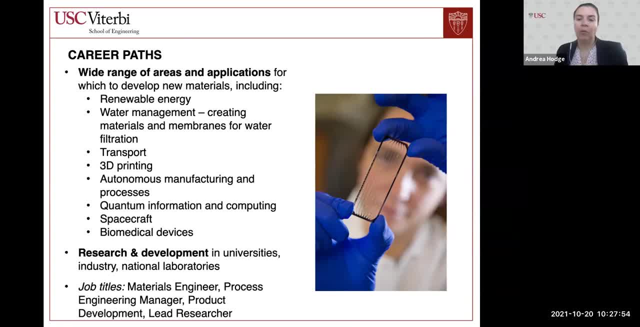 what to say workforce professor nomura and professor bachista. so we have a question here about coding experience to take these classes? um, and i know that we also in the selectives have a couple of 400 level classes which would be more introductory and still Part Programم. I think that might be part of the elective courses. uh, do they need to know coding or? 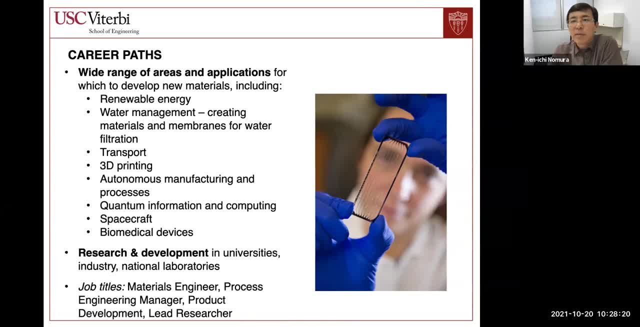 coding languages before they start the program. i think that's one of the questions that we see here. so so my assumption in like you know, 515 is: like you know, uh, people who have no, no experience of programming at all. so we would do it like you know, because that's, that's the kind of like our audience. 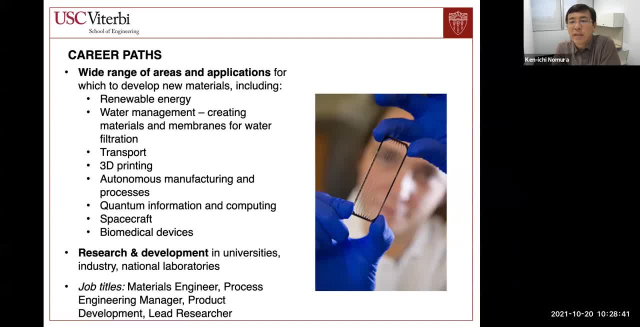 like you know, uh uh, we have our탁 him target audiences like materials engineering people who are interested in applying machine learning, AI technology to their field, But I think, because this is new field, so that many of them you have no experience- 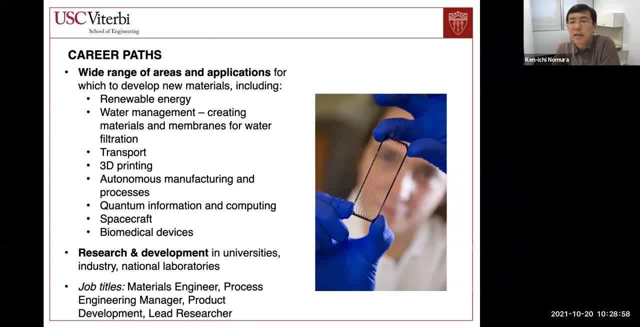 of programming or computer science algorithms. so we'll do it basically step by step, And also for the students who may have questions. so say: well, I will feel better if I take an earlier class than these three core courses. Like I said, we do have some 400 levels that are also based on both molecular dynamics. 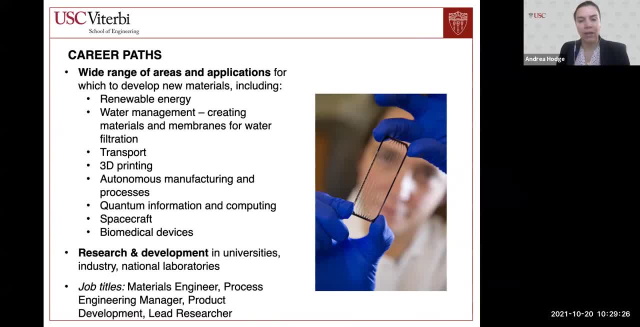 and machine learning tools that are taught by Professor Bacista and those can be approved as part of the electives and you can always take those before you take the core courses if you feel. that will be better, although it's not necessary, And also for those students who are 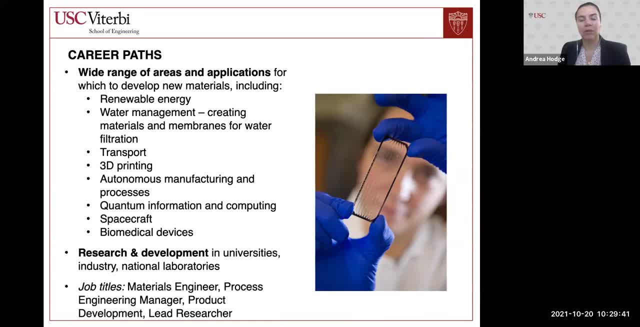 Are USC and want to do a PDP, that may be another, A progressive degree program. that may be another way, another route to enhance those skills. Again, I think Professor Nomura said it wonderfully: this is Our target audience is people with materials science, materials engineering background. 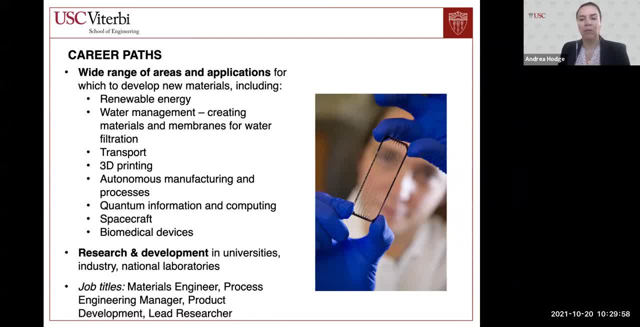 who want to then learn about machine learning. So there's no prerequisites about your computational skills, although you will have to learn those in order to earn a master's in materials engineering with machine learning. Yeah, I see another question here. I'm not really sure: is this a paragraph in the degree that? 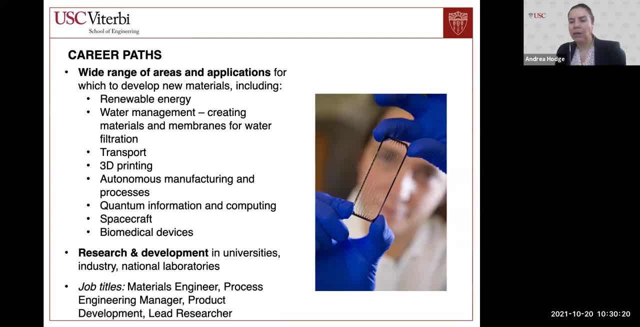 you can either do it in materials science or mechanical engineering. So these master's program is in more family department. it's not in mechanical engineering, but you could take a lot of electives that are cross-listed with mechanical engineering, but the degree still will be from. 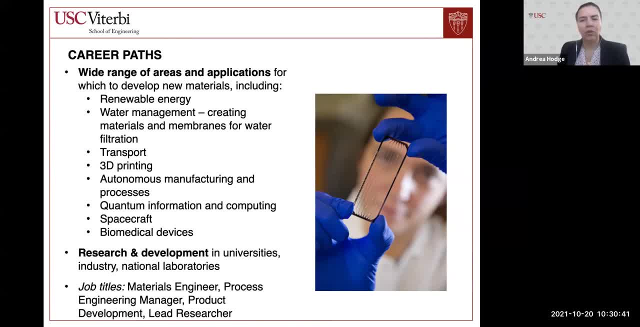 In materials engineering. So I'm not sure if I'm answering that question correctly, but it's not a mechanical engineering degree, it's a materials engineering degree from the more family department, But those electives that we saw in there there's lots of classes from mechanical engineering. 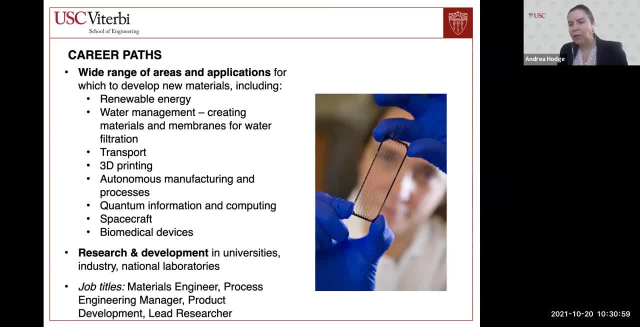 that can be cross-listed. So hopefully that kind of answers that question, or, if you can be a little more specific, I think we can aim to provide more specific answers, Okay, And I think that, if I can add to that for this question, if you are wanting to take, 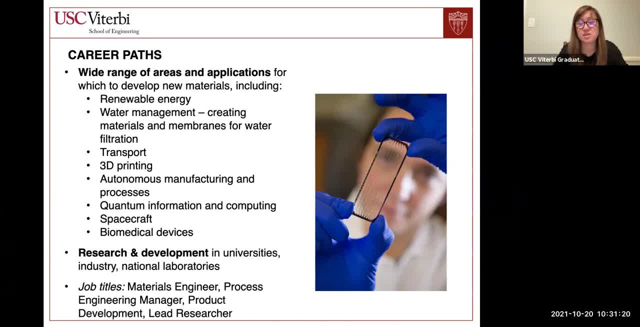 courses from the aerospace and mechanical engineering department. it's kind of just a matter of meeting with the advisor in the materials science and chemical engineering and petroleum engineering department to be able to just get that approved. So I think if that's your question, in terms of getting it approved, that would just be. 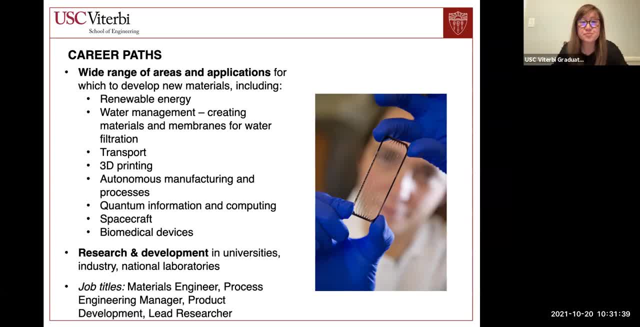 a matter of meeting with your advisor. Okay, And the same thing. if you're in another department and you want to take these core classes in machine learning, you can also do so without having your degree in our department. So there's that, because there are such listed as electives and they can be approved by speaking. 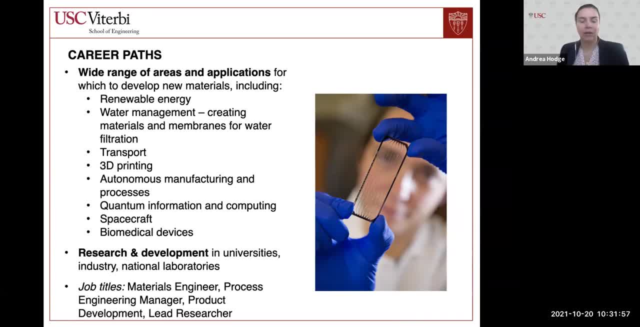 with your student affairs advisor in your respective department. So there's a lot of flexibility to really tailor the master's program to what you're interested in and what you want to do and what you need. Okay, Thank you, And then perhaps we can just give everyone just the last couple of minutes to ask any 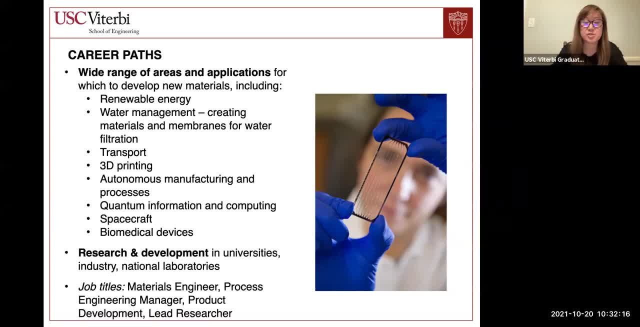 remaining questions of our professors. And if you do have questions about applying and admission and things like that, I'm happy to kind of stay on. but just in the interest of time I like to respect our professor's time because I know they're busy. 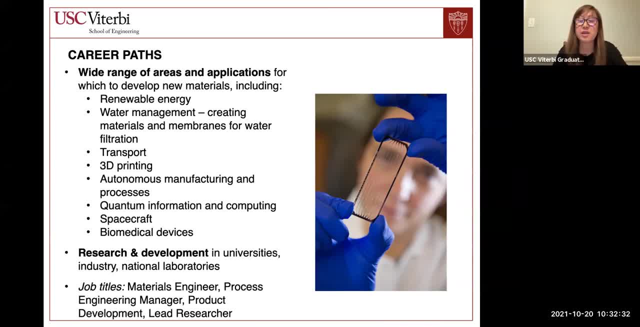 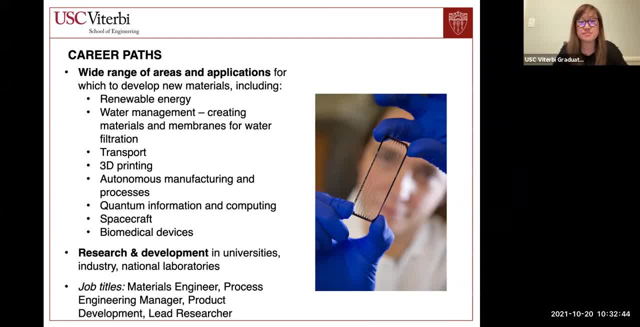 Yeah, sure, I mean. I just want to say as a faculty member in the department and as an experimentalist- because I am not in a computational group, my group is a fully experimental group- I am recommending these master's program as part of my PhD students doing a master's in. 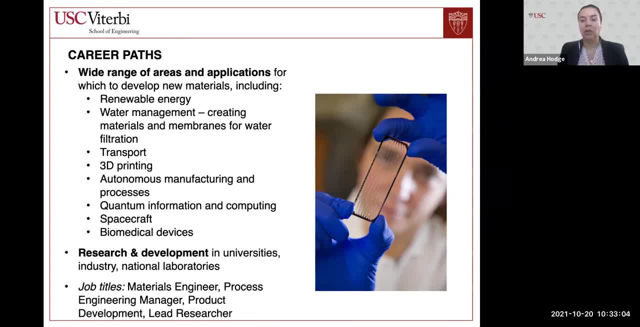 machine learning and the PhD in material science, just so that they have those skills so they will be more competitive the job market and also because it will make our research process more efficient by using data science and machine learning tools for again, for the faster materials discovery. So 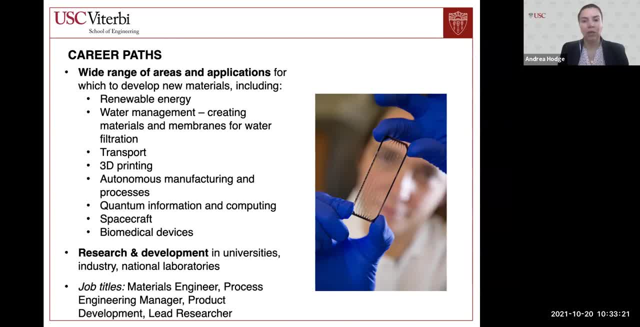 if you don't necessarily want to go into more computational route. there's also a direct correlation on how these master's program can help you build a better and more effective experimental career. This is where the future is going in materials science, and this will be what 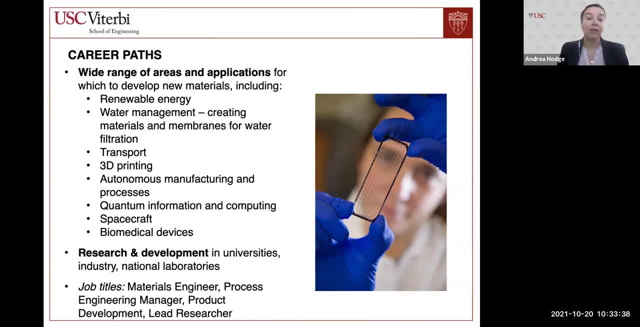 I would be recommending to all my incoming PhD students to take. They will be taking these three classes and part of these master's program in order to enhance their skills and be more competitive and be right now having the edge amongst all the other materials science departments across the. 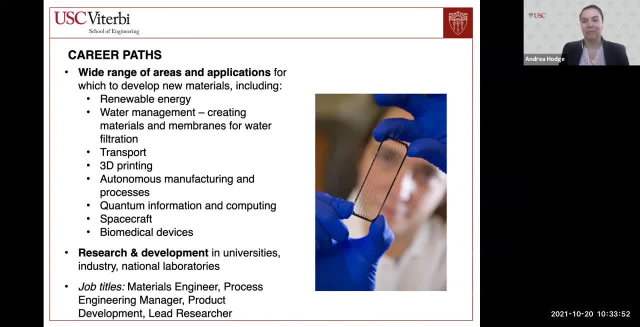 country. Thank you so much, Professor. I'm going to go ahead and put my contact information also in the chat if anybody has any questions after the close of this presentation, but it does seem like perhaps The questions are probably subsided at this point. Okay, Okay, So we have recorded this session.